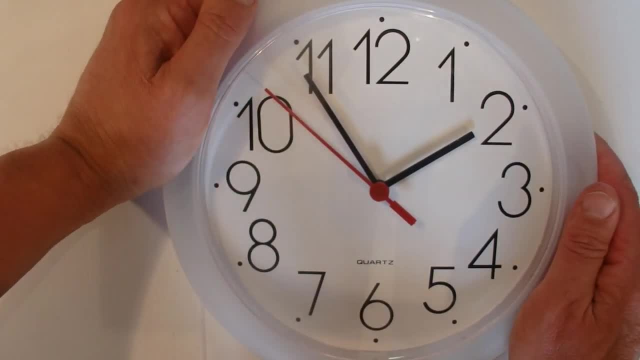 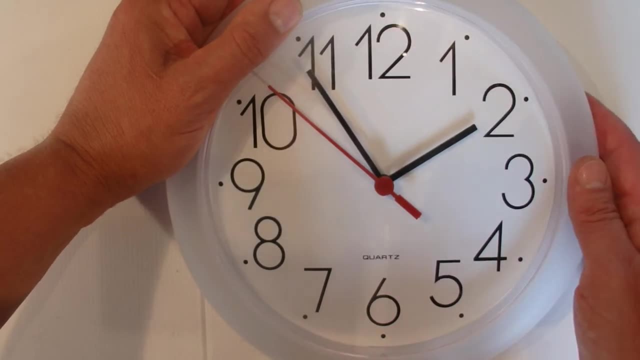 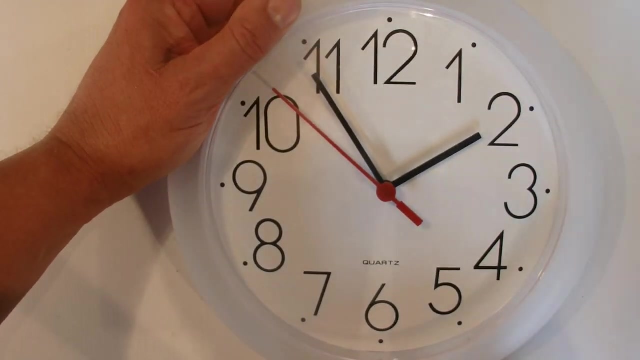 Otherwise I'm going to go straight into the answer, and I guess the obvious answer is that you know there's 24 hours in a day and the hands appear to be making right angles twice every hour. so two times 24 is 48. so the obvious answer might be: they line up 48 times. but actually 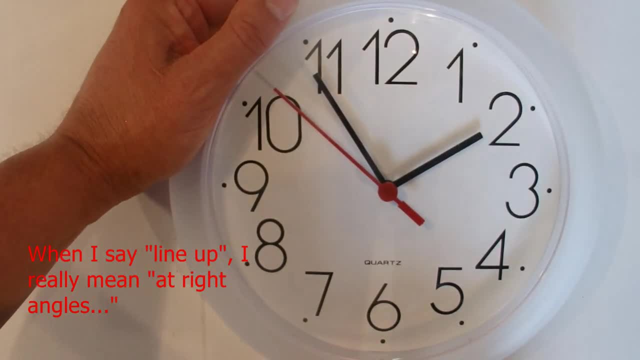 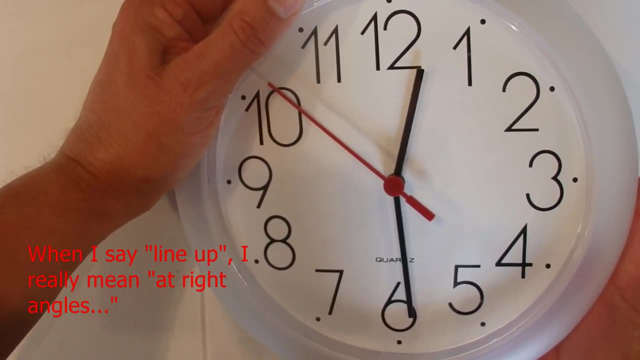 they line up a little bit less than 48 and actually line up 44 times. and I'm going to show you why. Think about the first time we saw the hands make right angles in a 24 hour day. So the hands on the clock line up. sorry, the hands on the clock made right angles. it was at 12.16 and 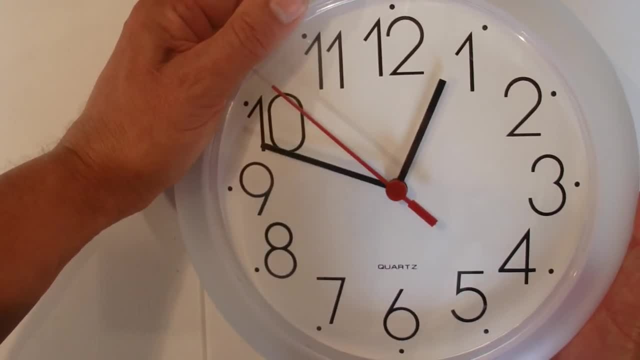 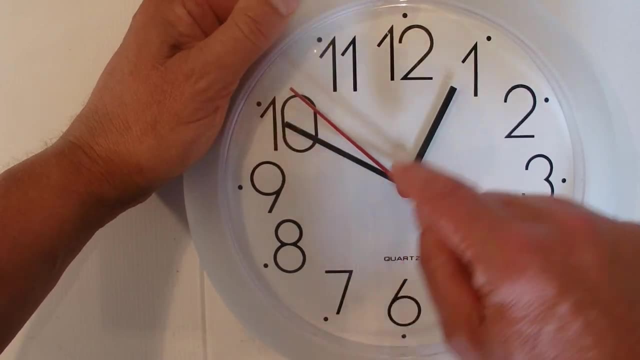 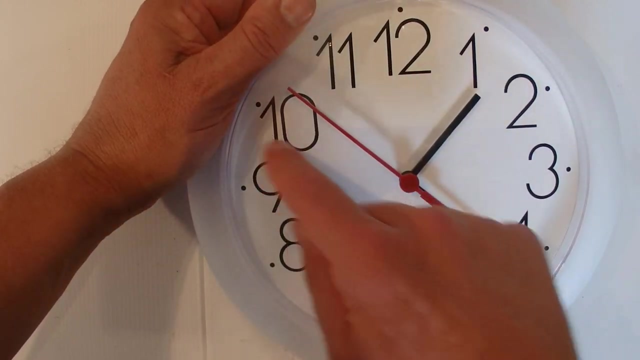 the next time they made right angles it was actually at 12.49, so it wasn't exactly half an hour on. it was actually about 32 or 33 minutes. on that they made right angles the second time, and then the third time they made right angles was around here at 1.21, and that also was around. 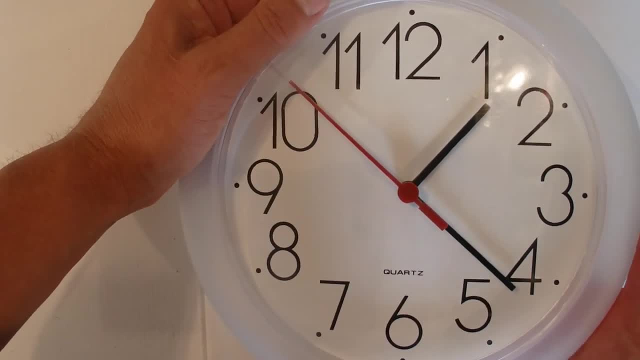 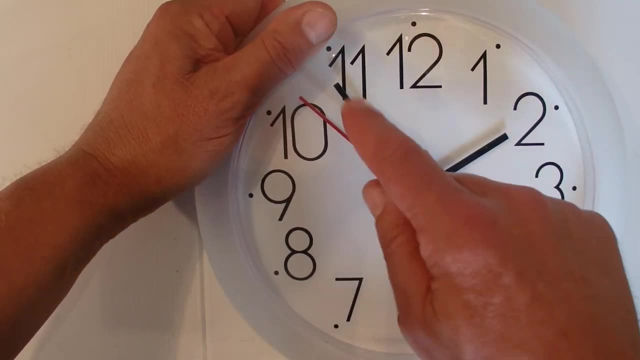 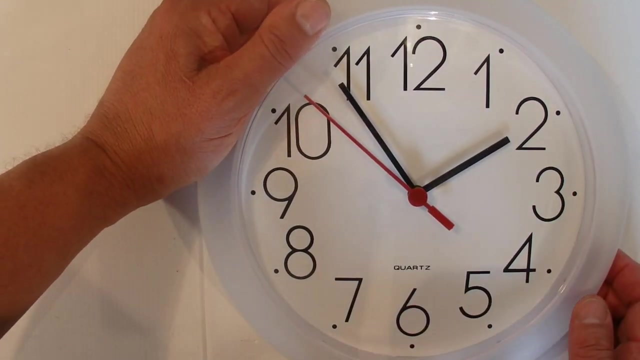 about 32 or 33 minutes on the clock minutes on. The fourth time they made right angles was around here at 1.54 and it also wasn't exactly half an hour. it was actually at 32 or 33 minutes on and I guess when you 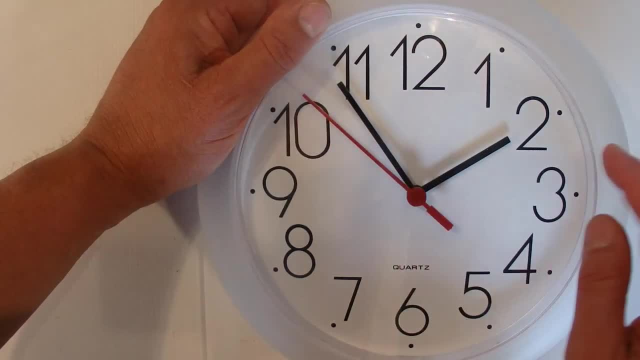 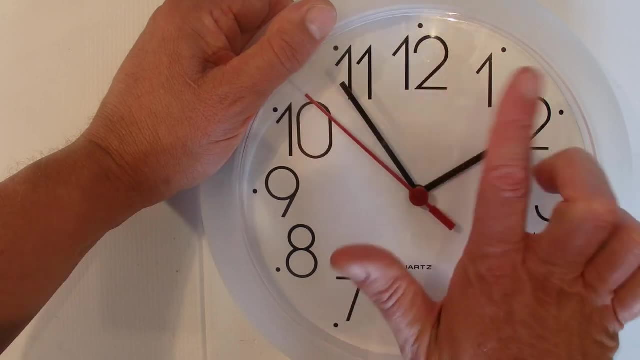 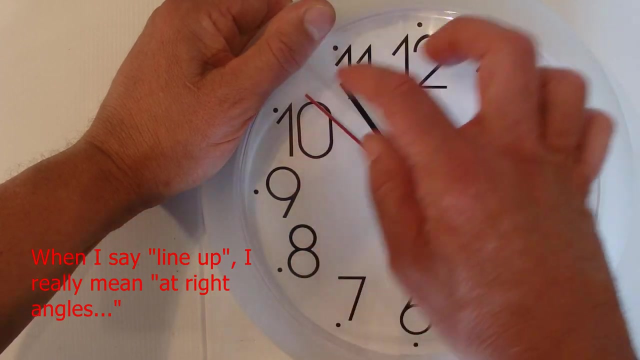 think about it: in a 24 hour day that there is only roughly about 44, lots of 32 minutes. so if they are lining up every half an hour exactly, then you would have 48 in the 24 hour period. but because that is an extra few minutes every time they line up, then that adds up. 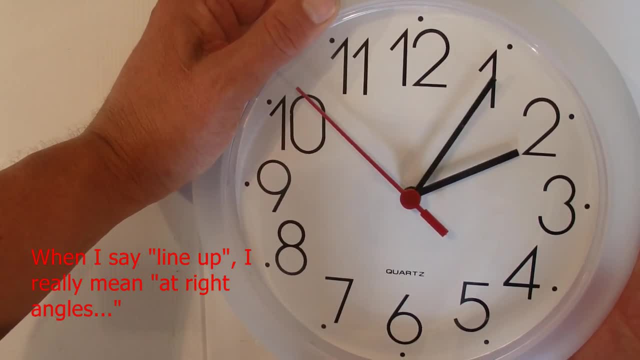 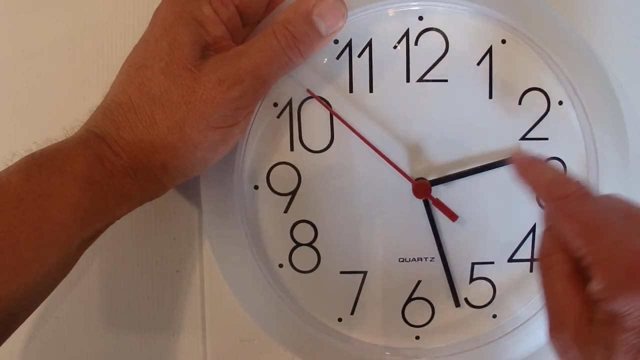 and you have only got 44 times that the hands are at right angles in a 24 hour day. This is obviously when you get to the 2 o'clock range, because the first time the hands make right angles in the 2 o'clock is at 2.27, and then the next time they make right angles. 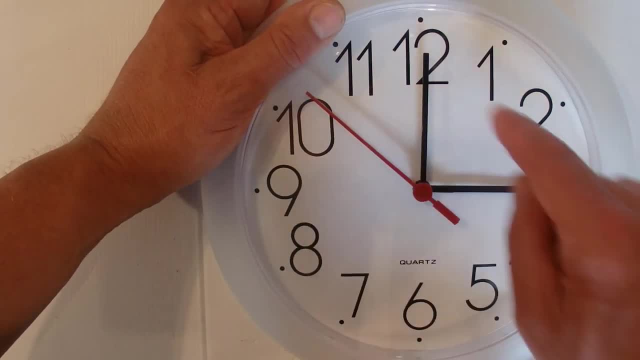 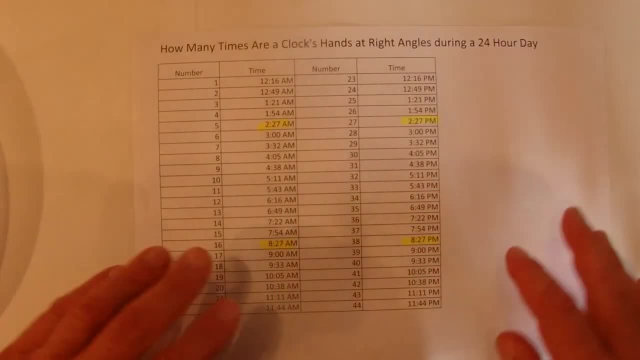 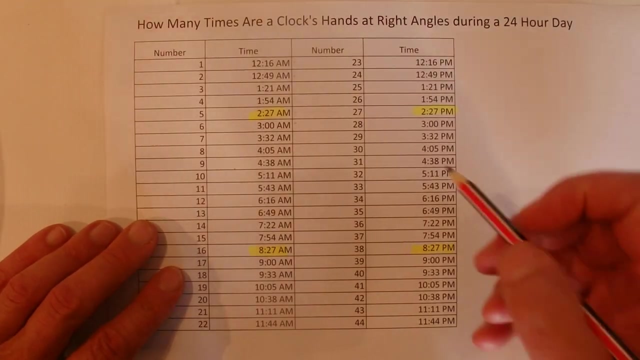 is at 3 o'clock, So there is only once in the 2 o'clock range that the hands make right angles and I have done this simple little grid so I won't go through every combination because it will probably take too long. and a simple little grid that shows all the times. 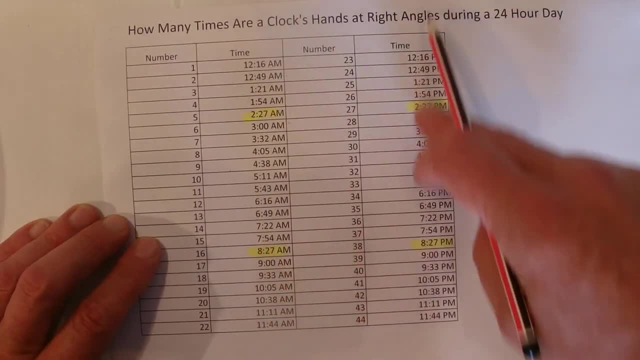 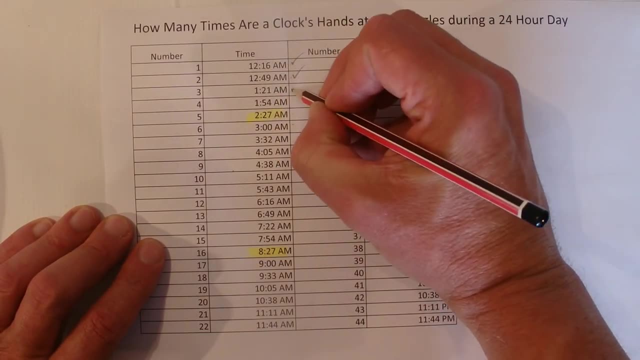 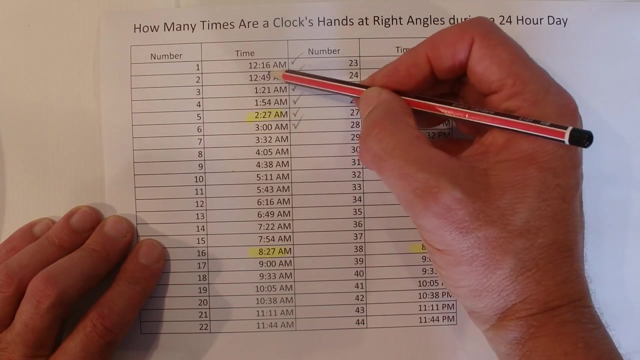 that the hands make right angles in the first twelve hours and then in the second twelve hours. and if you think about it, oh, they are the ones I have shown you: 12.16 and 12.45, 121,, 154 and 227.3, and you can see there that the, the the times are advancing on. 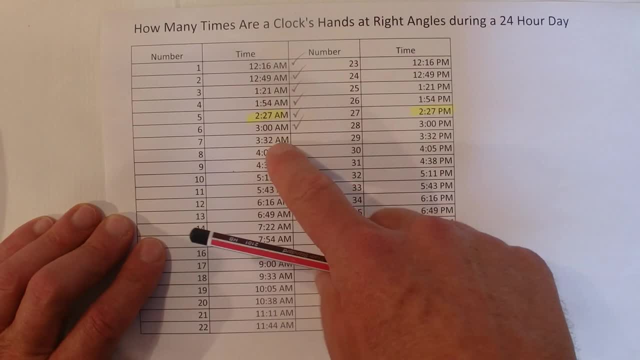 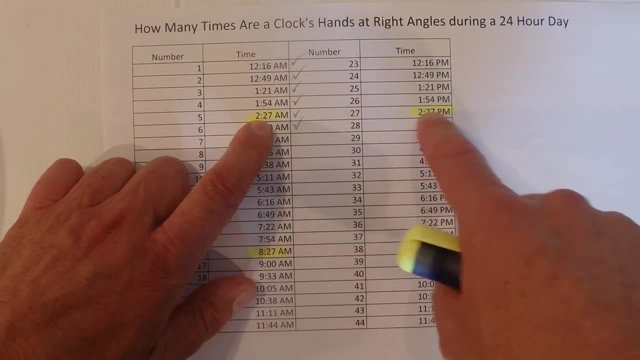 around 32 or 33 minutes every time to when they make right angles, and I guess it's obviously in the two range, because in the two o'clocks then the hands only make right angles once in the two o'clock, both in the morning and in night. 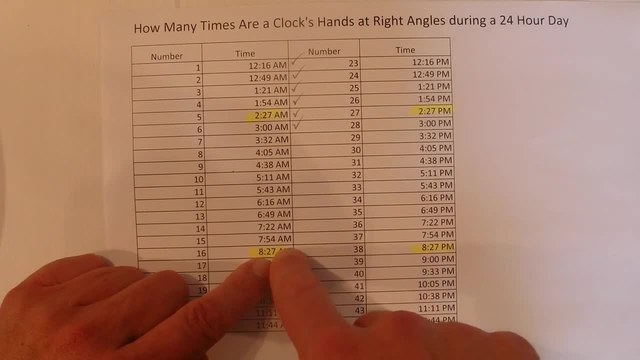 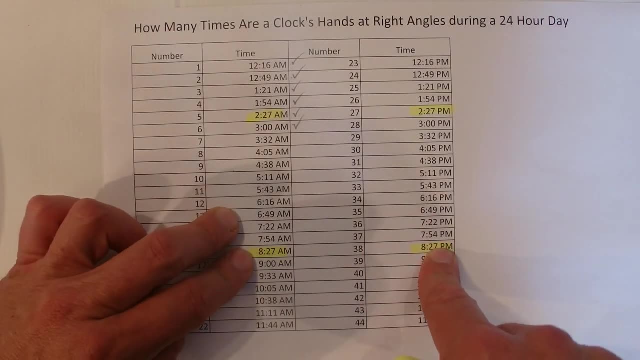 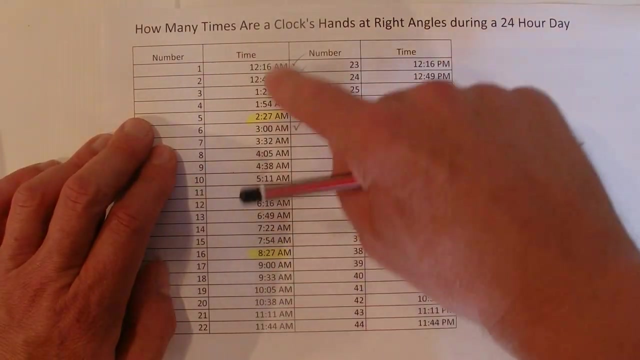 and also down here in the eight o'clock, that the hands only make right angles once in the eight o'clock, twice in the sevens, twice in the nine, same in the evening, but only once in the eight o'clock. and you can see there that all those times that the hands make clocks, hands make right angles 22 times in the. 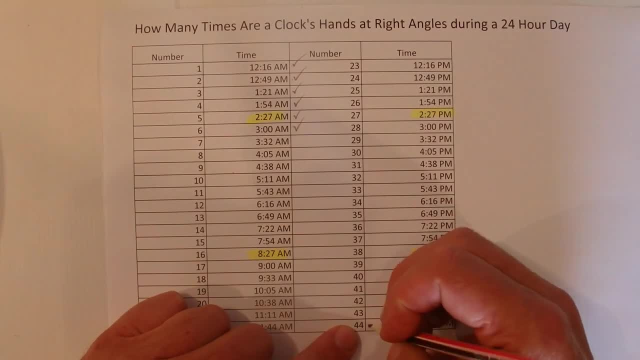 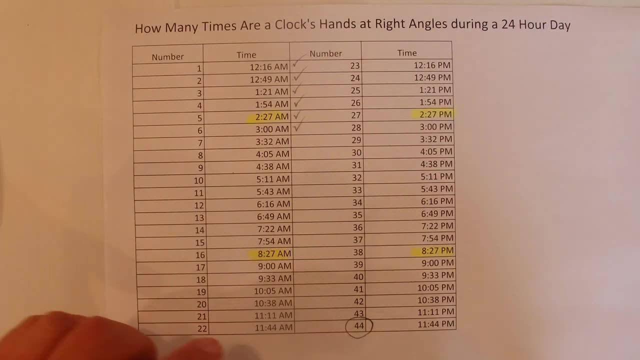 morning, there's another 22 times in the evening, which leaves with a total of 44 times that the hands are at right angles in a 24 hour day. okay, well, I hope you've enjoyed this video. thanks for watching and goodbye for now.